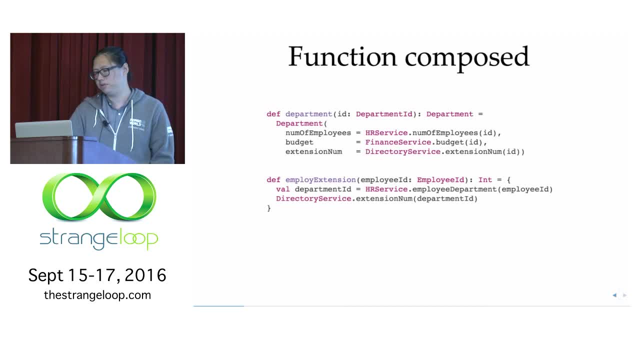 So very simple and everybody knows how to do that without any help from cats or Scala Z. You just build a function that give an ID and you build a new department. The problem is that you have bound variables right. I mean we are doing functional programming. 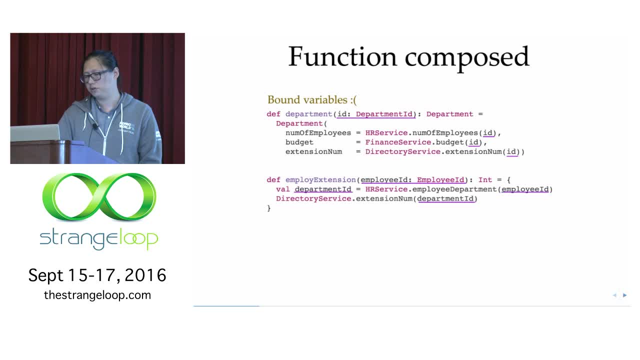 Why do we need all this? First one: you have to pass it in, Hold all the services and get a value out And then put them into a department. The second one you can create: You have to first call the employee department function, Then you get a department ID and then you call the directory. 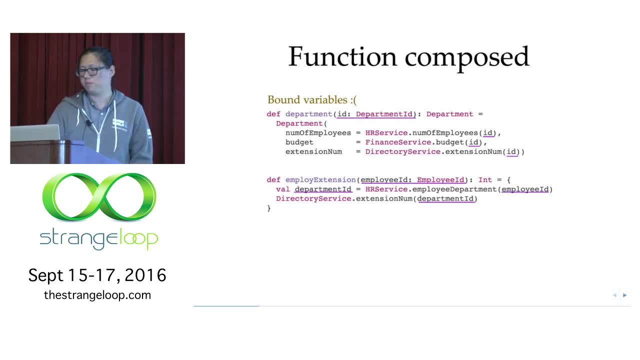 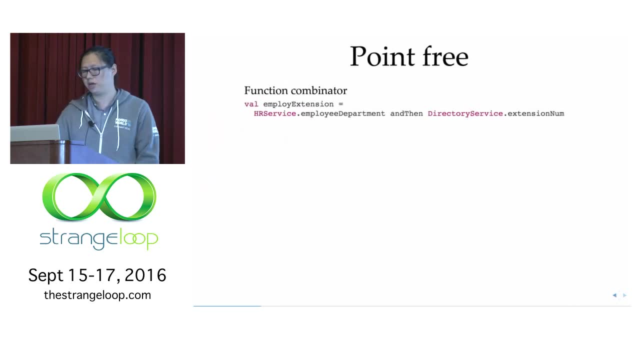 service extension number method to get the extension out. So we know better, right, We can do functional Function combinator For the second example variable to get an employee extension. we can just combine the two functions and then you just have two functions combined and you get one function out. You don't have bound. 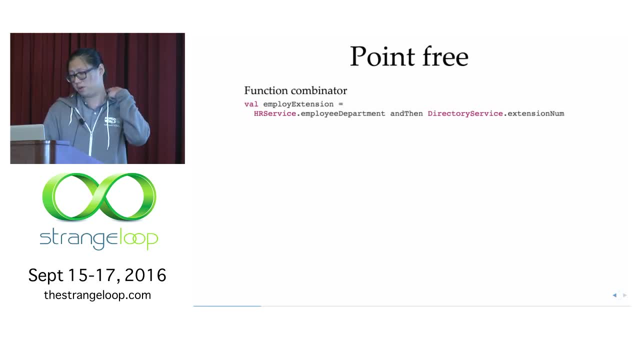 variable. It's just going to be employee extension. You call the employee department first and then you call the extension number next. That's it So great, Awesome. What about this one? So you have now. this one is a little bit tricky, right, You're? 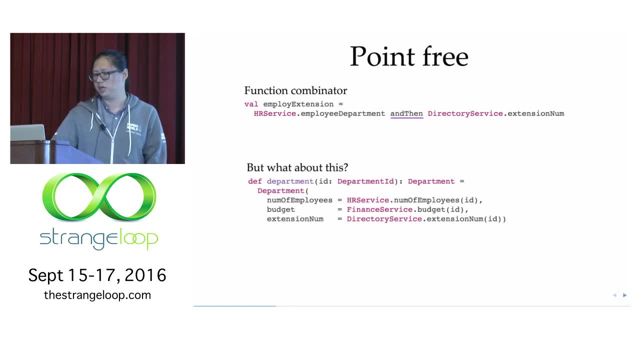 basically trying to have: you have three functions and then you have a department apply function. The three functions that you have all takes the department ID, which is simple, but the department case class apply method takes three different elements. I mean arguments. So okay, 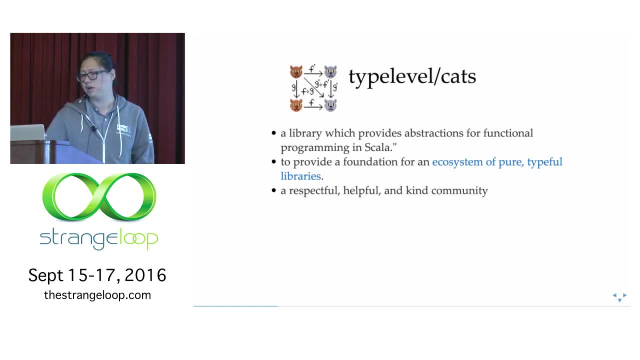 So then here's what CATS can provide. The first thing that CATS can provide for you, first introduce CATS. It's a library that provides abstraction for functional programming in Scala, Okay, Okay. So it also like trying to provide a foundation for ecosystem of pure type for libraries. 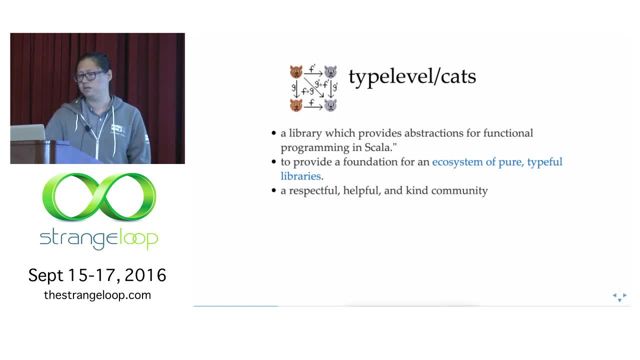 They have I think right now dozens of libraries built on top of CATS And also one of the important goals for CATS is to provide a respectful and helpful, kind community. It's trying to provide really help for doing functional programming in Scala. So with CATS the first thing that 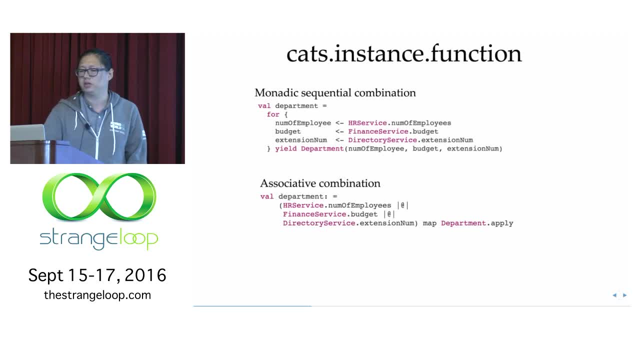 we can do is say, okay, function actually is just a monad, CATS provide a monad instance for function, applicative instance for function as well, so that, as you can see, we can do monadic sequential combination. So the first one just say okay for all of these functions. 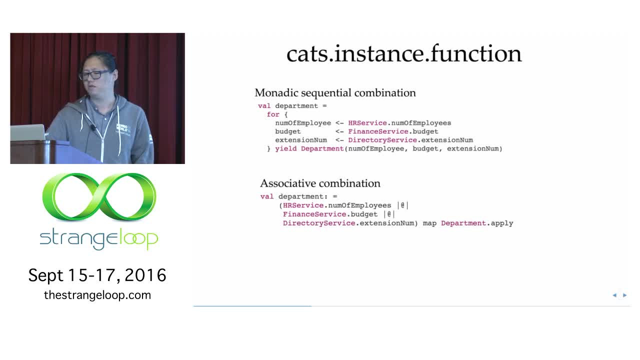 we just use, like for loop, a monadic for loop, and then we get the department out and that's the function for getting the department out. Okay, Okay, Okay, I'm glad you have that. And then the first thing you can do is say, okay, function, actually is just a monad, okay. 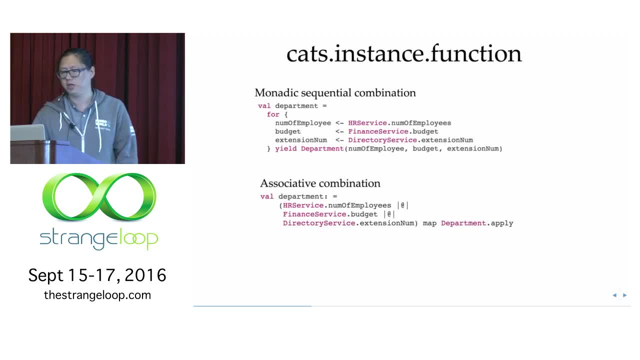 for getting a department. You don't have bond variables anymore. And the second one is the one that I actually could probably want to use at this particular scenario, which is associative combination. You just use the apply and condition builder to build three functions. use the tie fighter combinator to combine the three functions together into 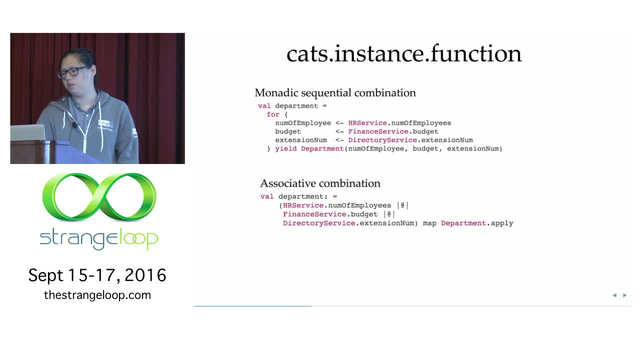 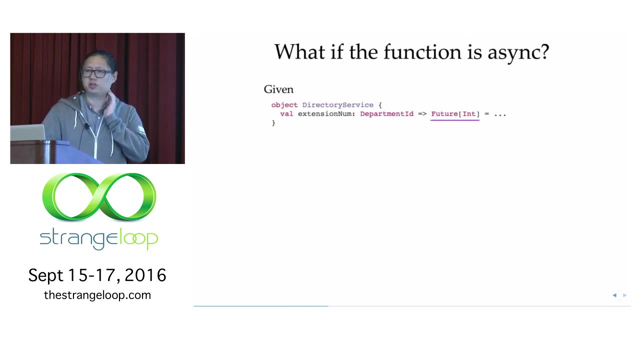 a condition builder and you map that into the department apply method function And then you've got a department function that takes ID and then gives you a department. So that's awesome. Yeah, cats can do that. So what if the function is asynchronous? The 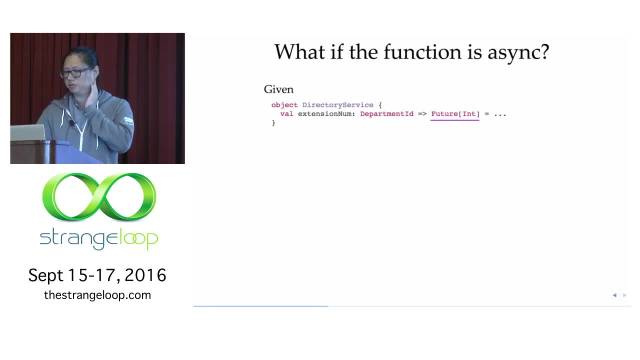 function no longer returns just the value, It's just no longer blocking, It returns the future of integer. So in that particular case, do you fall back to how many of you will fall back to bond variable? Nobody Cool. So you probably all know the trick. The trick is cats has this thing called classly. 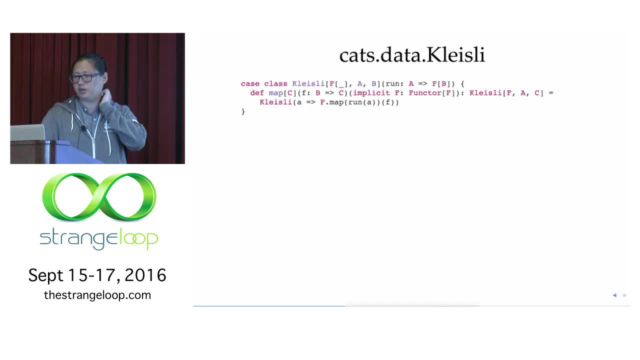 but it's a typical functional programming thing that you can wrap a function which does not. It's a function from A to B, and instead of a function from A to B you take a function from A to F of B and then you can do all kinds of things with this classly. 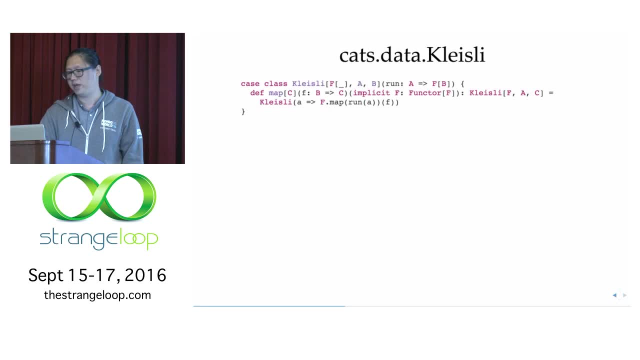 combine them, compose them, And then you canwirtschaft from A to F of B, and then you can do all kinds of things with this classly and combine them, compose them, and compose them, and then you can transpose them just like they are a function of A to B. So the example we see here is that 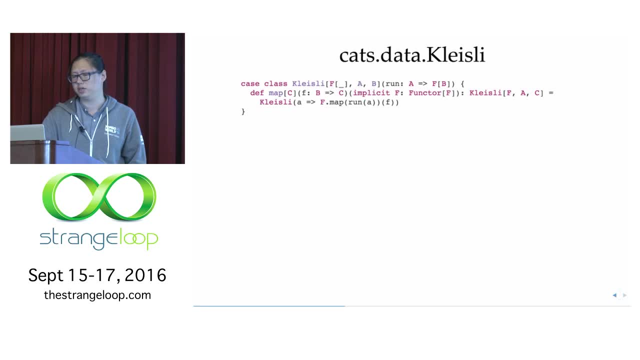 you can map right and map this classly and you can create a. you have a classly from A to F of B and you have a function from B to C and you map it. you got a classly from A to C. So that's just the same thing as you map a function. 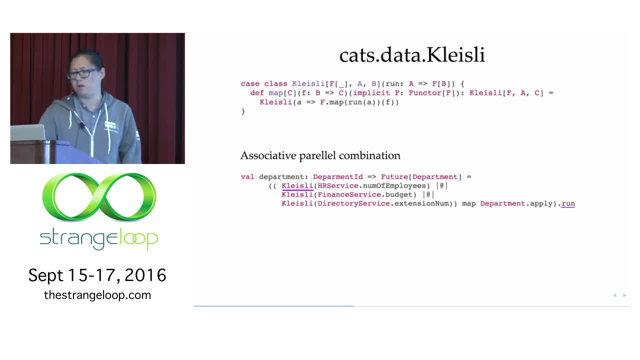 So then we can do the combination again with this class with the help of classly. right. We can say: for associative parallel combinator we just wrap, use the classly, wrap each function and then for each classly it's an objective. so we can just do the same combination. we. 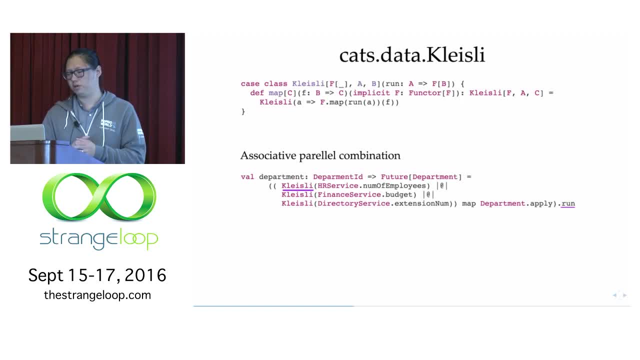 did before, which is use tie fighter to you know, congregate them together and then build a bigger condition builder and the map to the deployment apply, And then you can do the same thing. So then you can do the same thing. 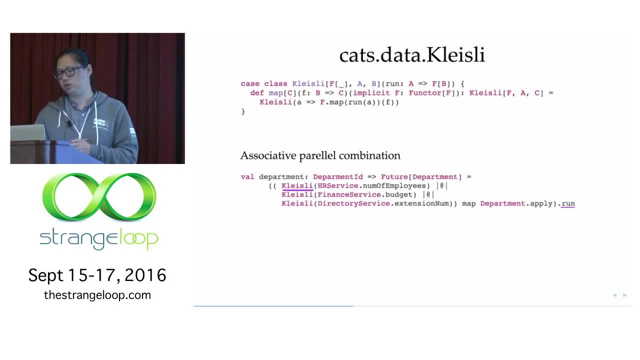 So then you can do the same thing. So then you finally get a classly out of that and you call the dot run method of the classly. As you can see, the dot run is just the field on the top here. It's just the function that classly contains. 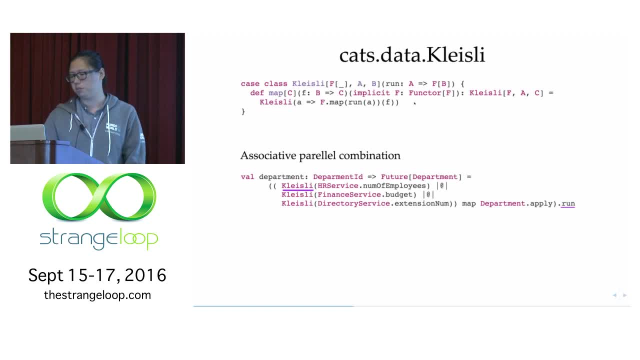 So you unwrap that. you got a function from department ID to future of department. So that is neat And then you can also do and then So classly has this method that helps you do and then So you can do the sequential combination as well. 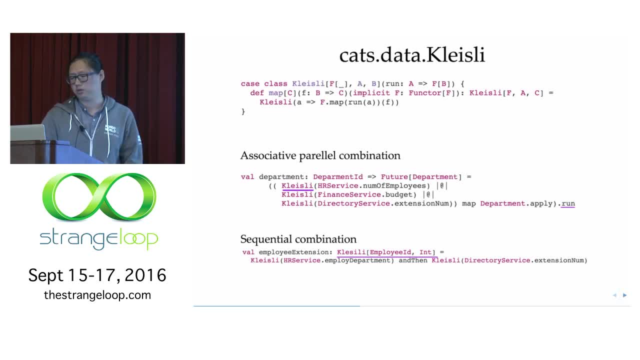 So you do have this function and then you can do the same thing. So you have the, and then combination between two classlies and then you got a classly out which is. so the two classlies you have is a function from for employment department. 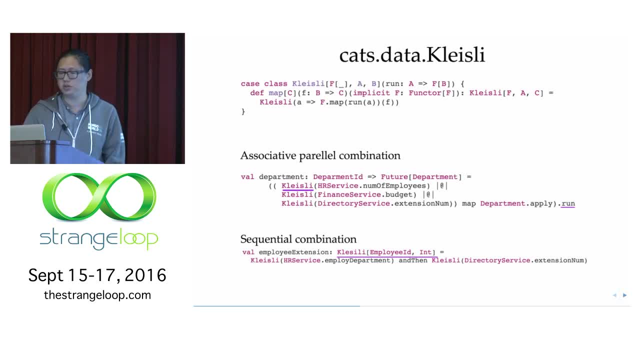 you get a. you basically have a function from employee ID to department ID and then you have a function from the department ID to extension number and you just call and then and then you got a function or classly from employee ID to extension number. 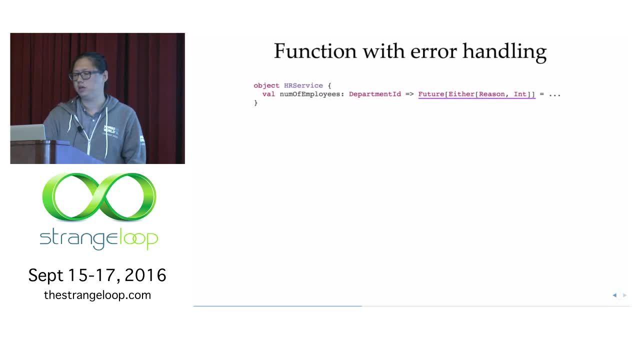 So okay. So then What if your function has error handling right? So we just keep making our function more realistic. Error handling with future is actually already baked in, So you can just use the futures baked in error handling, as most of the case. 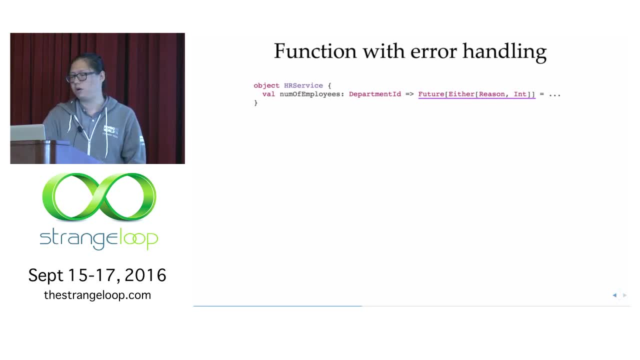 But in some cases we want to use either to do error handling You want. in this particular case, I can see I use a reason on the left of the either side. That's the reason is. This could be just the ADT, where I have the full list of all the possible reasons that 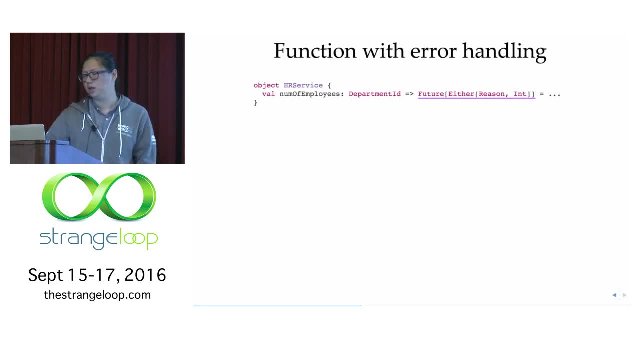 could cause a program fail and because it's ADT, I can make sure that I handle all of them when I handle them. So that's the beauty of, that's the convenience of using an ADT for your own error handling instead of using exceptions, which is what futures does. 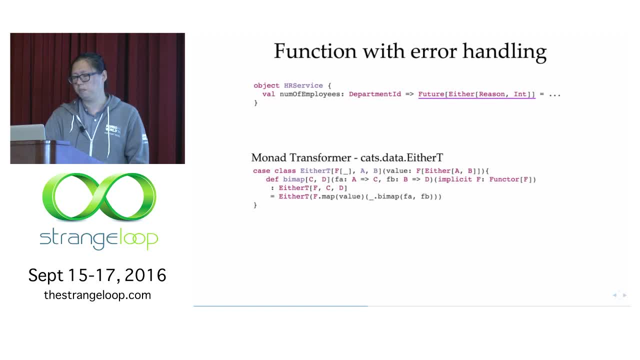 So what do we do with that? There's this thing called monad transformer, provided by CATS, So it's called IZRT. used to be XRT, but in the latest CATS we introduced IZRT, So with IZRT, you can treat the future of IZR as this thing called IZRT, which is a 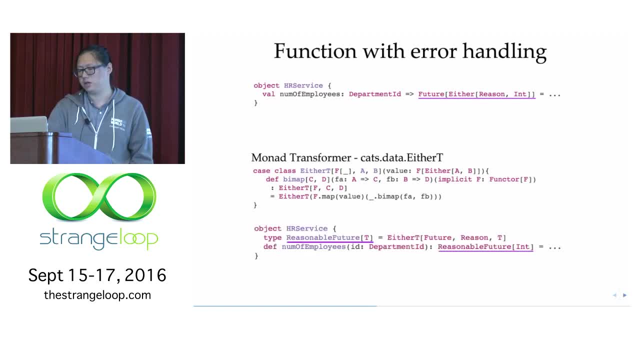 single monad. So then let's look at the HR service. If we have this type, we have this IZRT of future of reason of T, we can just create a new type called reasonable future of T, And that thing is just IZRT of future of reason. 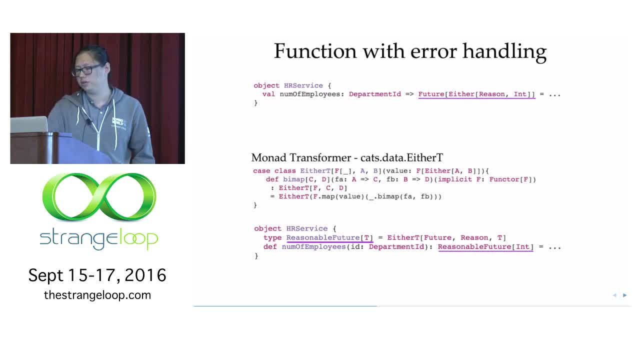 And that reasonable future is just a monad. And then, just like, instead of using future, you use reasonable future, which has this error handling big thing, Which is essentially just the future of IZRT, of reason and T. So with that it's the same. 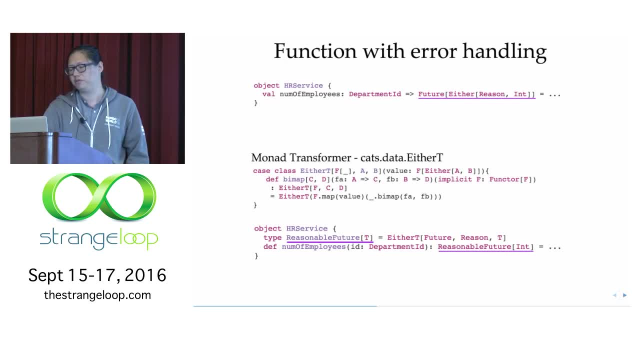 thing as before. We have a bunch of functions. instead of returning future of something, we return the reasonable future of something, But they are both just monads, So we can compose them the same way, using classly. So that's that. 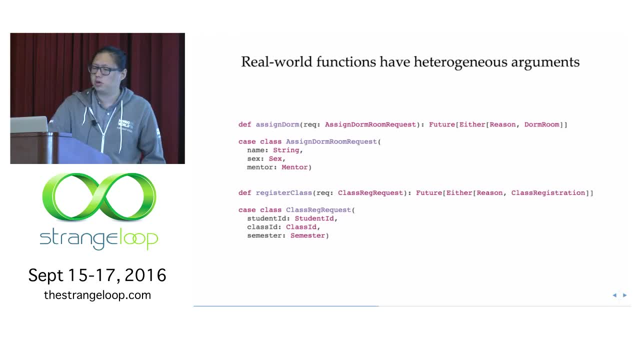 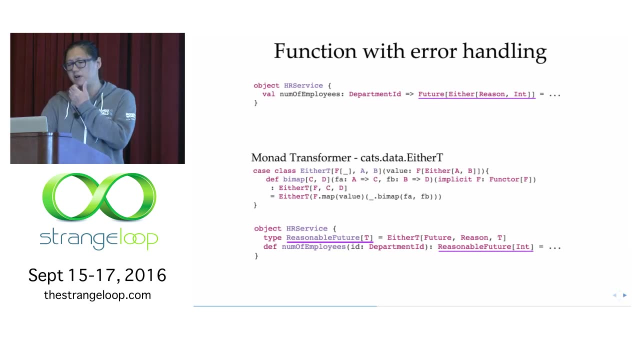 Okay, Now we go to the next level. So real word functions have heterogeneous arguments? They are not. The problem is this: The thing, The simplified things with our previous example is that they all take a single argument, department ID, And you know. but in real word you have different kind of functions. 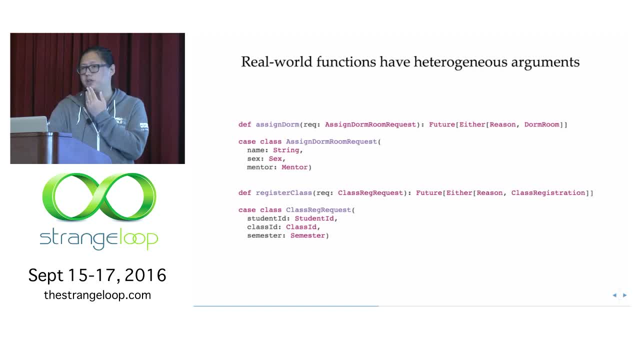 Each take different arguments and they have different data presentations, Like in this particular case, this particular example. you can see we have a signed dorm function that takes a request that has three digits. It needs three different fields, which is name, sex and mentor. 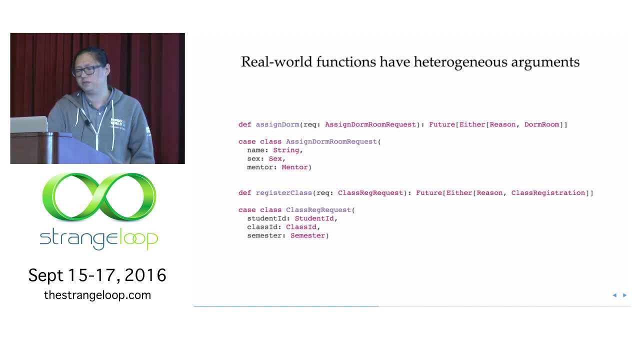 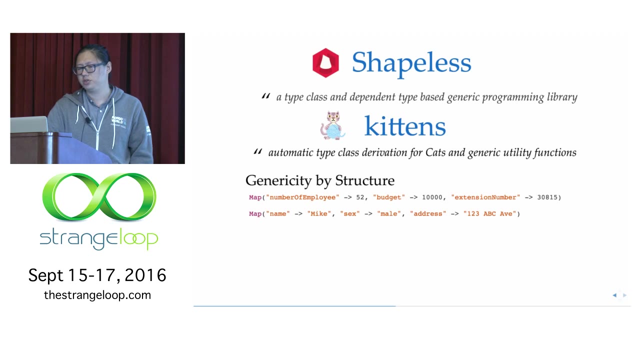 And we have a register class method which also takes different kind of data. So how do you compose those or combine those? That's, before we do that, we need to do a detour to introduce shapeless and kittens. So shapeless is a type class dependent type. 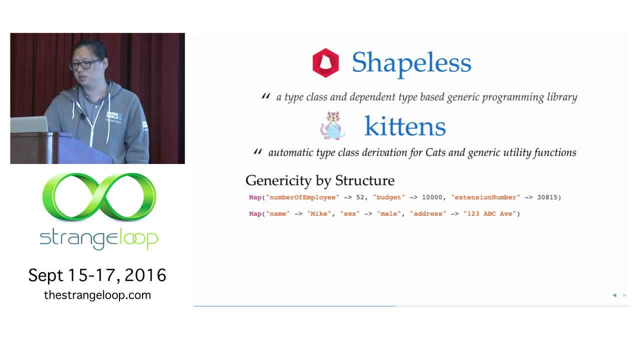 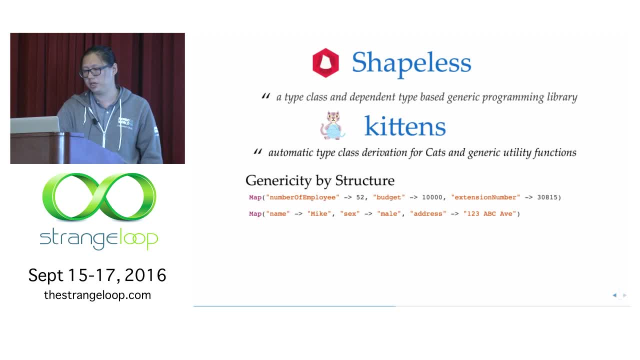 It's a type class. It's a type class. It's a type class. I can use an example to explain that. And kittens just build on top of shapeless and cats. So the example I'm going to use is: first, let's look at generosity by structure. 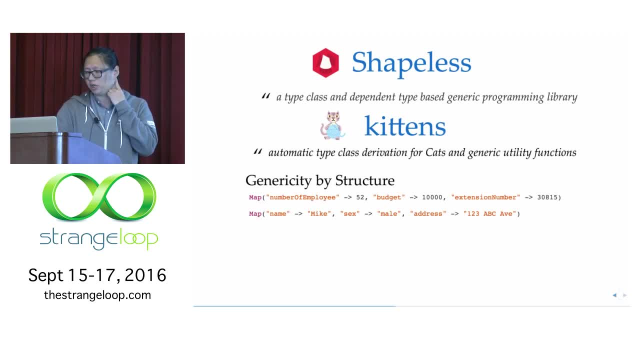 We all know maps right. The first map is a map between string- The key is string, The value is integer- right, And we know how to work with a map. We can map it, We can iterate through it, We can do all kinds of stuff with it. 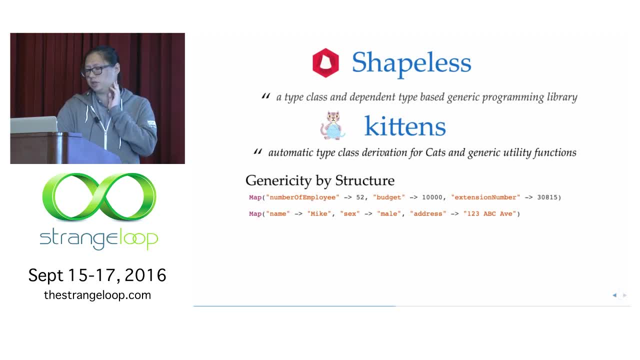 And the second map is a map From string to string. It's the same thing. We all know how to deal with a map. It doesn't matter how many fields it has, It doesn't matter how many items it has. We can do the same thing. 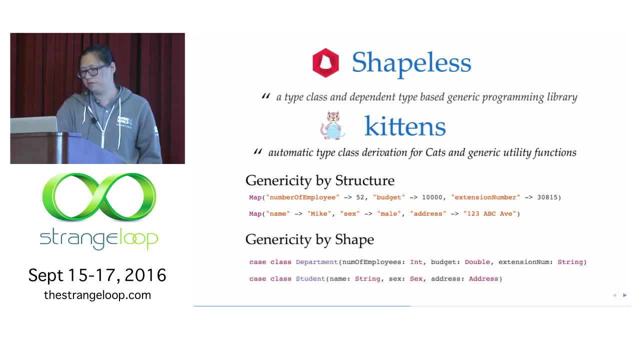 So what about generosity by shape? So we have two case classes, But if you screen it really hard it's just like my maps, But they are just different. It's called products, So they have data of different types. They just combine together. 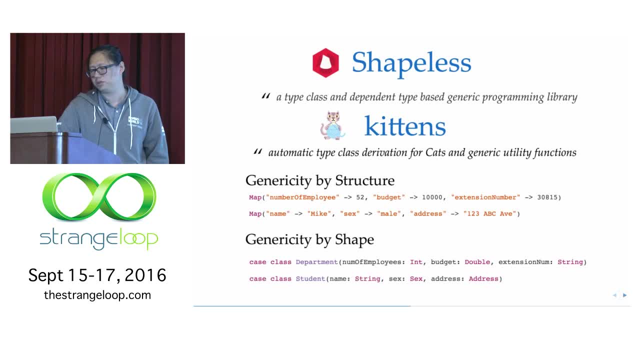 Each one. Say: the department has number of employees, which is an integer, or a budget, which is double extension. number is a string, But it's just a product, It's just a combination of several different data. So the same thing goes with students. 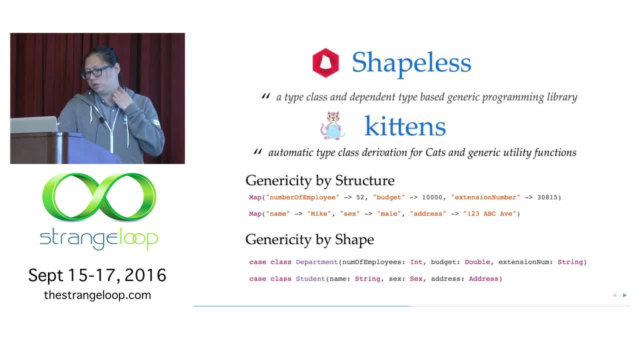 So the idea is that we shouldn't need to write a code that is specific to department or student. We should just treat them as we treat maps- Just the same thing. So let's look at it. Let's continue to look at example. 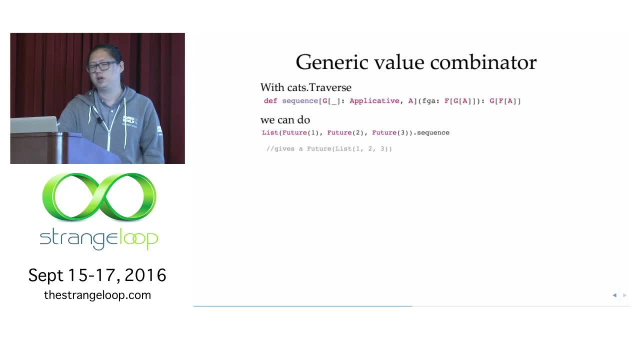 So for example, in CATS we have this type class called traverse And with traverse one of the functions traverse provides is called sequence. So if you have fga, which is f of g of a, and if that g has an objective instance, 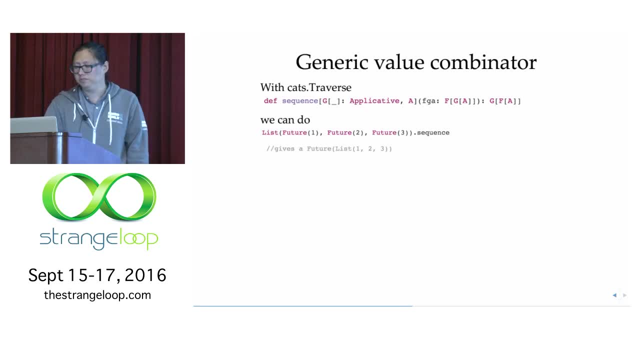 you can turn that into a g, of f, of a. Well, that's abstract. So a concrete example is that you have a list of features right, a list of feature one, two, three. You can sequence them into a future of list- one, two, three, which is a lot easier to work with right. 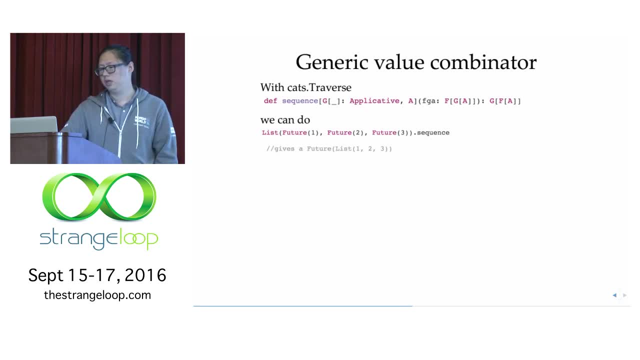 That's cool, But what if it's not list? It's this thing, It's this department, case class, It's a product, right? You have three different items of different types. So you have this code that you just extract them out and construct a new department. 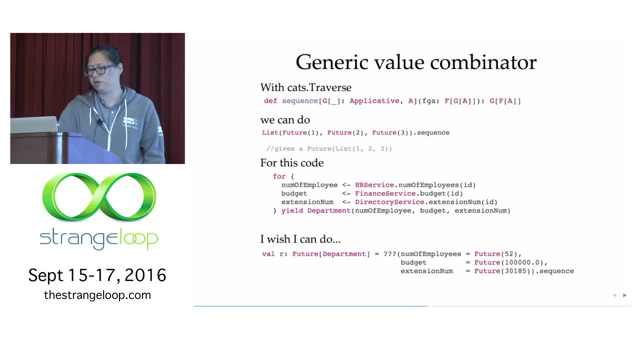 But I wish you can. what you can do is just say: you know, number of employees is this feature, but is this feature an extension of this feature? Let's just do a sequence and we can sequence out a feature of department, right. 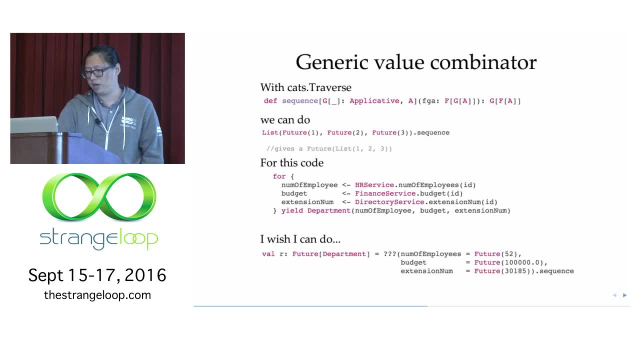 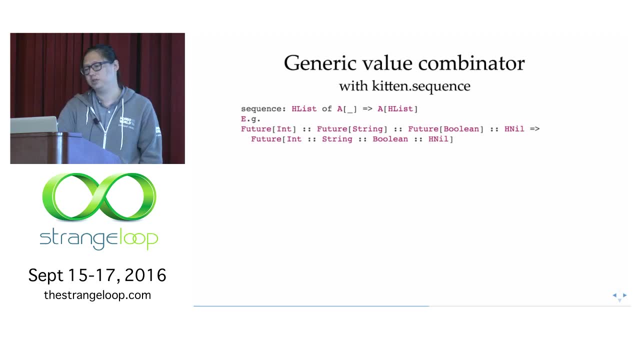 That's what generic value combinator is about. So basically, CATS has this functionality called sequence. exactly as you're thinking, It's sequence against a heterogeneous list, an H list. So basically, if you have an H list of A, which A has a collective instance, 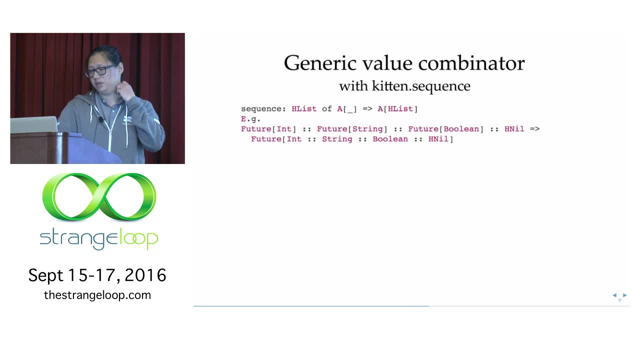 then you can just call sequence and it give you A of the H list. So a concrete example will be a feature list of a feature of A and a feature of string and a feature of boolean And you just call sequence and you got a feature of H list of into string to boolean. 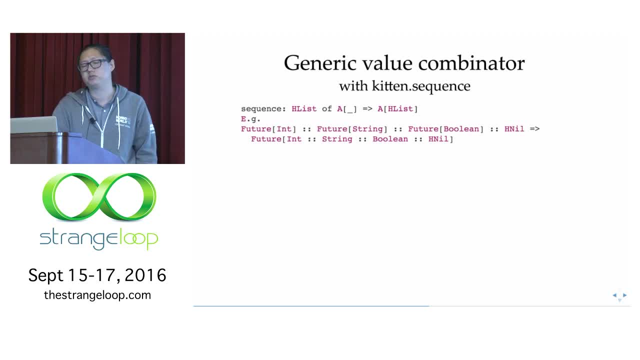 And that the last thing is just a new. it's just you know, the same way you construct a list, So let me see how long I have. So basically, we're back to the code that we just had, The. what we wanted to do is say, if I have a number of employees, a feature, a budget feature. 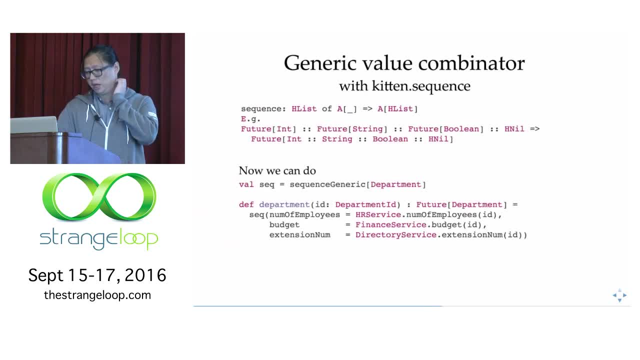 I want to just call sequence and I get a feature of department and that's exactly what sequence generic encadence give you. So you call sequence generic of department that give you this. you can say it's a combinator, so that you call this combinator with number of employees of you know, a feature of integer. 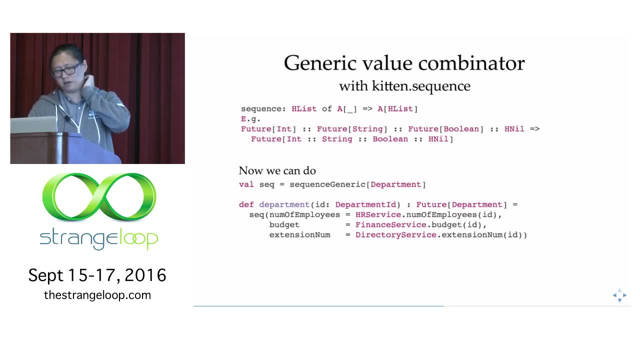 and then you call: budget equals the feature of a double and you have: extension number equals the feature of extension number. You call you give that to the combinator, It combines that into a feature of of department. Does that make sense? 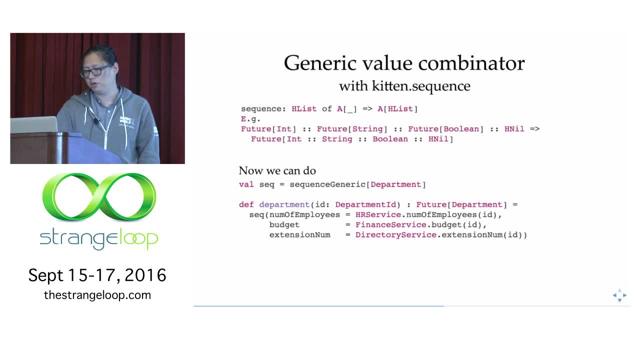 Cool. So now we can see. potentially this can help us to deal with the combining. how do we combine functions that have heterogeneous or different argument types? right, I mean this, give you something of that And you can see. but before we do that, 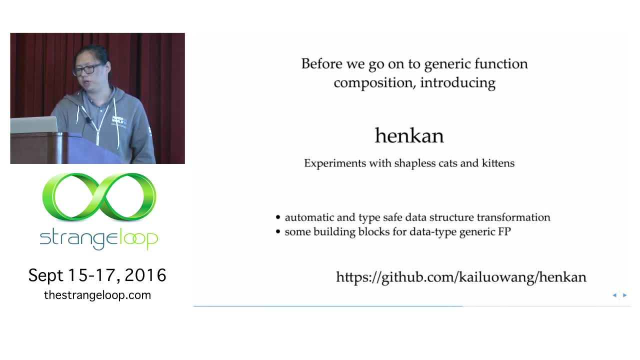 we need to just introduce Hankin a little bit so that we can introduce our more realistic example. Hankin is basically a very, very tiny library that are just a bunch of a cup of experience based on shipless cats and kittens, So it has automatic and type-safe data structure transformation and some building blocks. 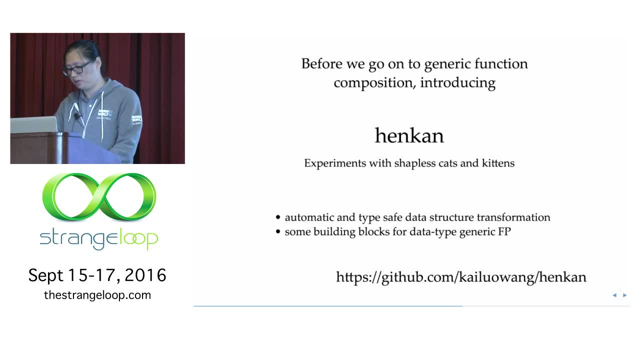 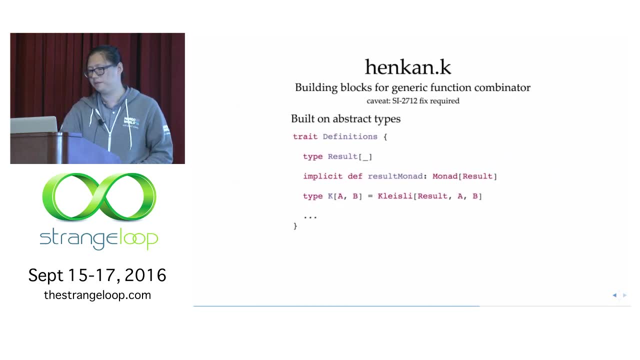 for data type generic functional programming. So let's take a look. First we have to define some types. So the whole idea of Hankin K module is- this is one of the modules Hankin provides- is to provide a building blocks for generic function combinators. 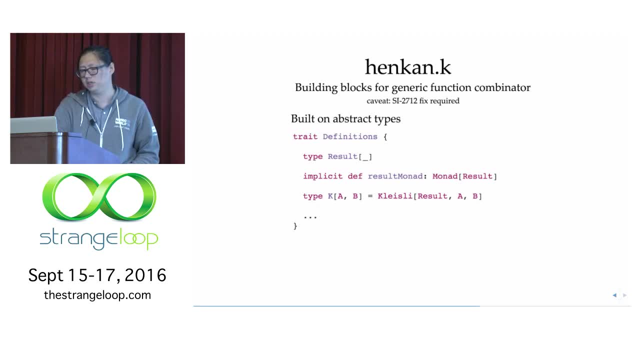 And the core idea is to do that using a classly, And so we've start with some type definition. We have abstract types, So classly must have a so-called result monad, or you have to provide a type called result. 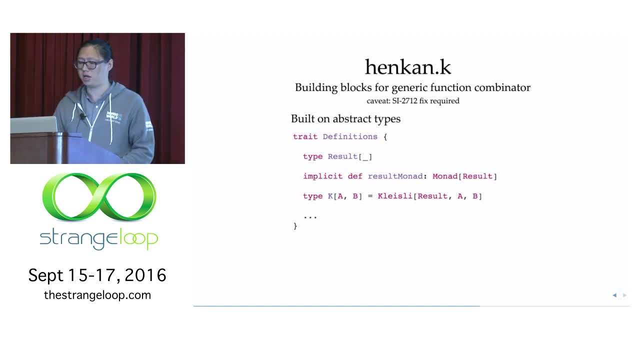 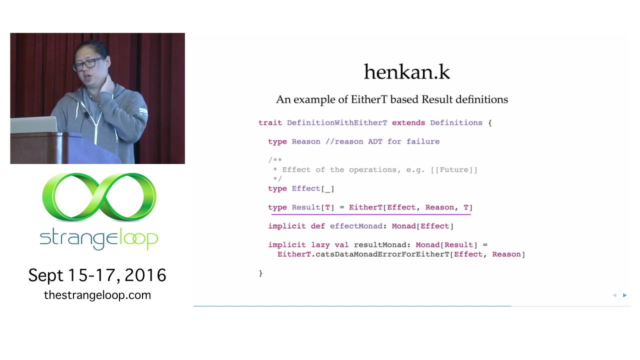 which you also have to provide a monad instance for it. but the result can be anything. So then you basically have this type called K, A to B. It's basically a function from A to a result of B. So to make that more concrete, we go next slide, which is we define the result to be IZRT of an effect and a reason and a T. 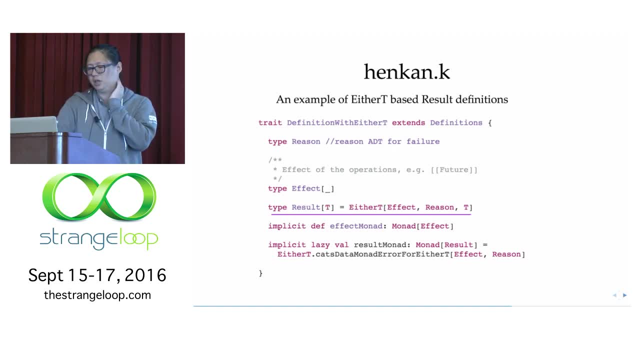 So this is just basically IZRT And the effect again is an abstract type, as you see above it, And there's also a reason. that is why the application fails. It can be ADT or failure, So this is a little bit more concrete. 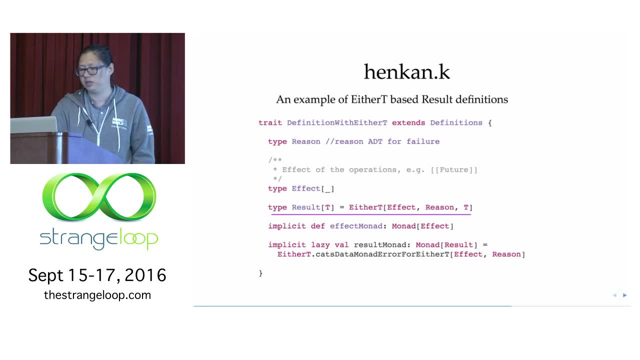 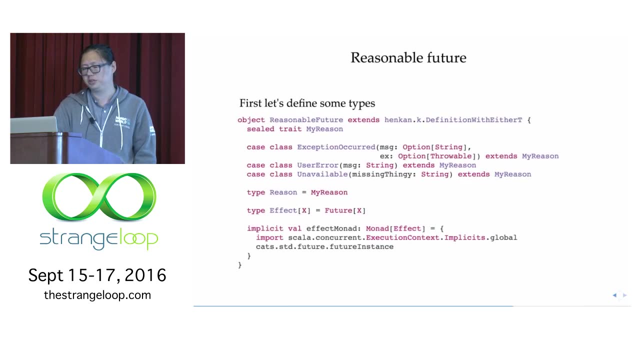 So you know the result is always the IZRT. So you have error handling there, but you don't know the effect and you don't know what particular reason is. So then the next. I can make it more concrete in your application. 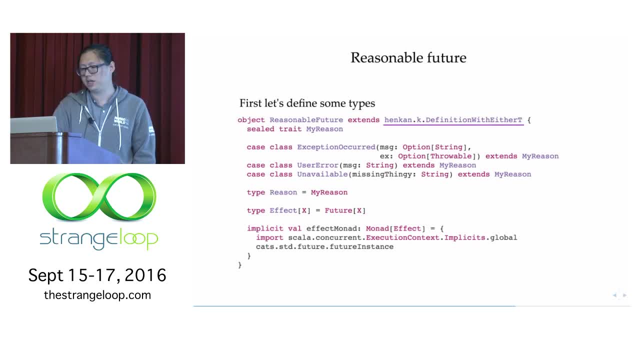 So you can say, for my, you just extend that trait and you can say the effect is just a future right, Just that type is just future. So it's asynchronous And for the type of reason you define ADT and this ADT, just you know, just a sealed trait in Scala. 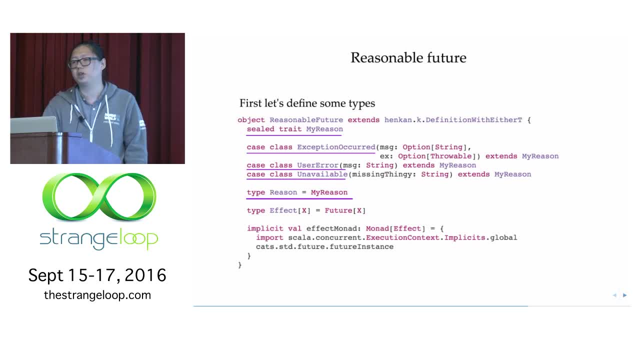 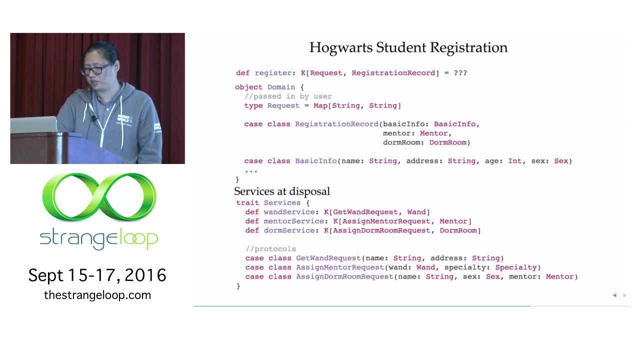 and you have a couple of possible reasons why application fails, like exception happened or user error or unavailable. something's unavailable, So you also provide an effect monad there. Now let's look at a realistic example: Hogwarts student registration. 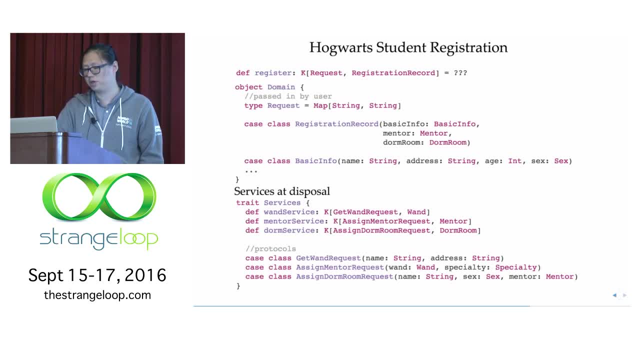 So this is quite some code here, but it's just business logic, so it should be pretty easy to comprehend. But say, I'm just trying to make it as realistic as possible, so bear with me. We have a type request. 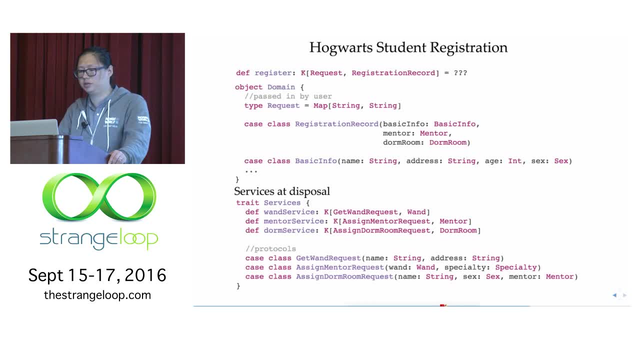 The first thing we want to build at the very top is we want to build a K from a request to a registration. A request is basically a map of string to string. This is passed by the user, so it's basically some random data, not random like the data input from a user. 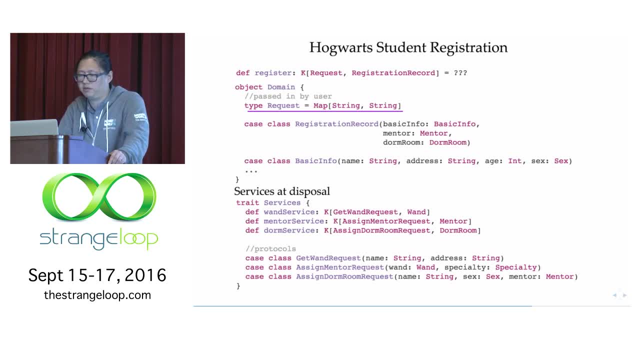 It can sync off as a representation of an HTTP request, whatever. Then you want to get this registration record out, which is some basic information like name, the address, age, sex. Then you need to assign the student a mentor. 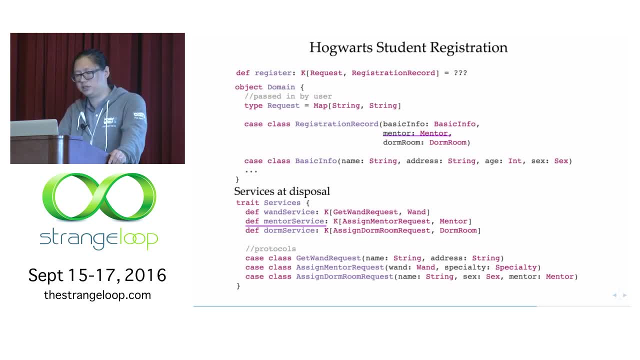 We use the mentor service to do that. The mentor service, as listed below, takes an assigned mentor request. This request needs several data. It needs a WAN. You always need a WAN to enter Hogwarts. The WAN is provided for you, unfortunately. 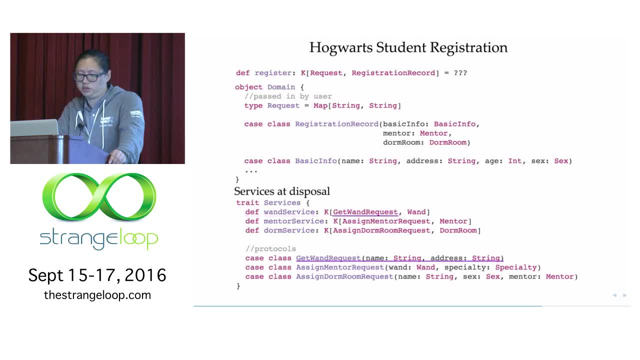 We use the WAN service to provide the WAN. This WAN service needs a name and address. That's it. Then the last thing it does is to assign you a dorm room. The dorm room service takes an assigned dorm request, which takes a name, a sex and a mentor. 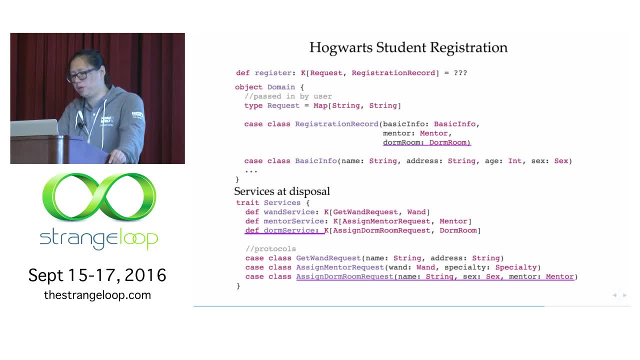 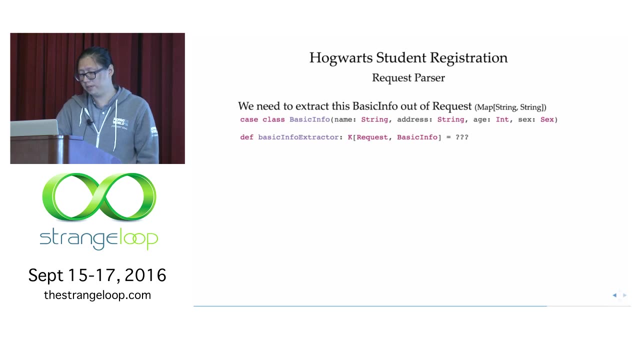 The reason it needs a mentor is that it then tries to make sure that people from the same mentor live relatively close to each other So that they can- I don't know- fight each other. So the first thing we try to build is the basic information from the request, which is a map of string, of string. 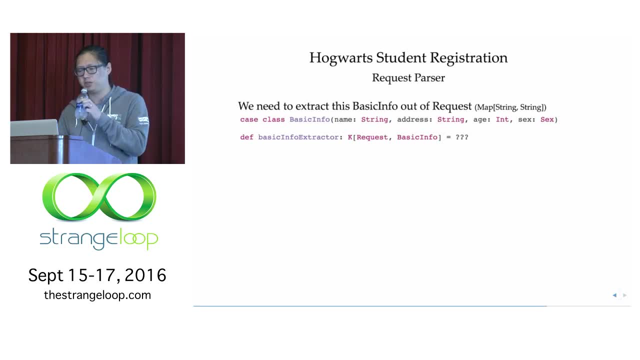 What we want to build is a key from request to basic info. Basic info, again, is just some data about a name, The name, the address, agent, sex. To do that, we first build an extractor, a K from request to string. 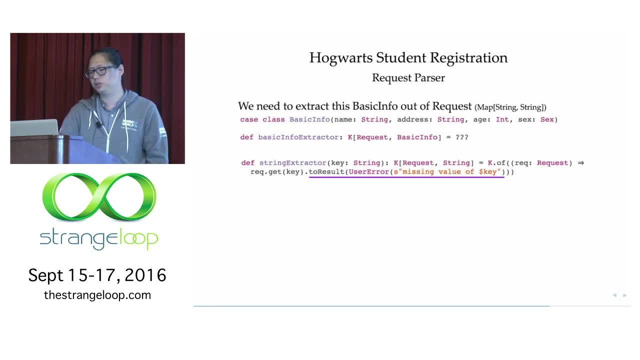 Request again, remember, is just a map of string to string. So to get a string out of a map of string, of string for a particular key, is pretty easy. You just say requestgetKey to result And the user error is just an error. 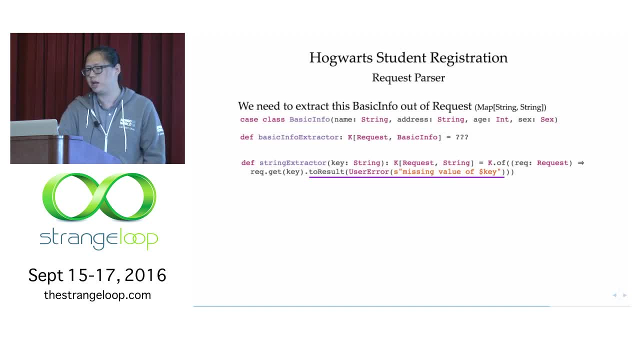 So when there's no such key in the map, we use that error. So that's it. The toResult method is a helper method provided by the. you write there yourself. It's basically when you say request or the mapgetKey, you get an option. 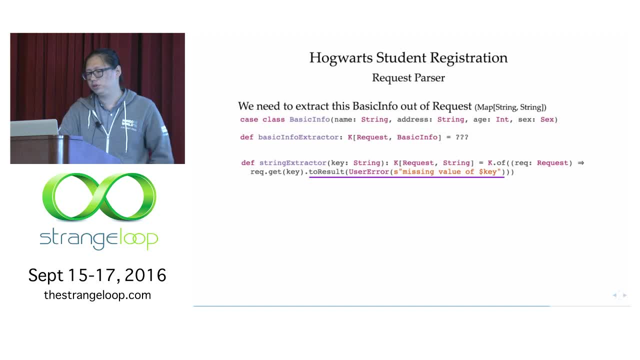 You want to turn that into a result which is either a future of either of reason or the actual string value. You call this toResult method. So cool, So that is easy to write. Now how do we get from there to extractor, from request to basic information? 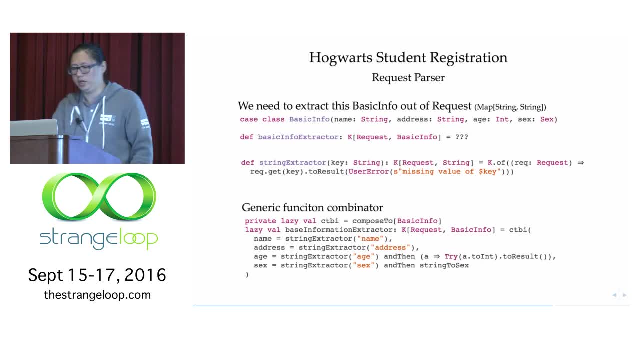 This is the generic function combinator as first introduced here. So you call this compose2 basic information. The compose2 is provided by Hank and Kay, Which is basically just using the kittensequence generic, And this one basically provides a CTBI. 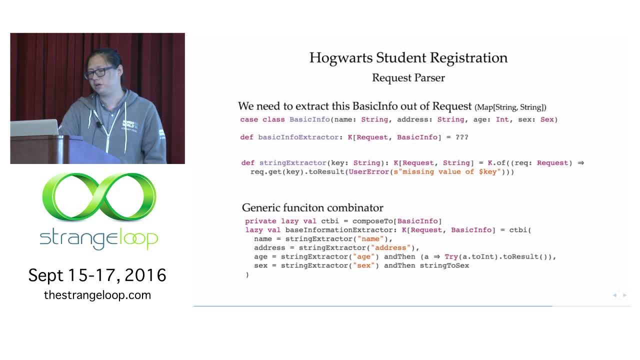 It's basically a function combinator to combine multiple functions or multiple anything actually into anything of basic info. So here's the example: If you have a string extractor of name, you can say my name is just the string extractor. If you look at the function above the string extractor name, just say: extract the value of under the key name out of this map. 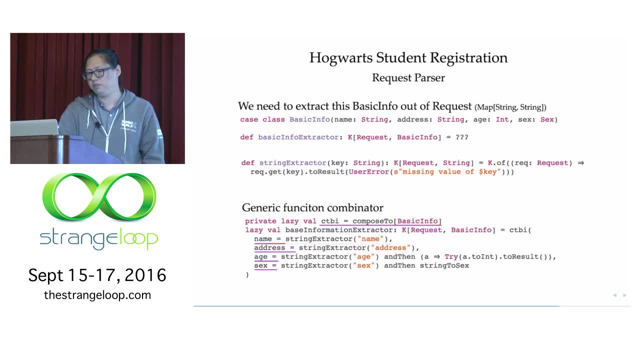 So that's just a K. So the first thing is just like name equals to this K of request to string, And the second thing is also that And then for age, we just call, and then for string, So our string extractor of age, basically extracting the value out of the age key. 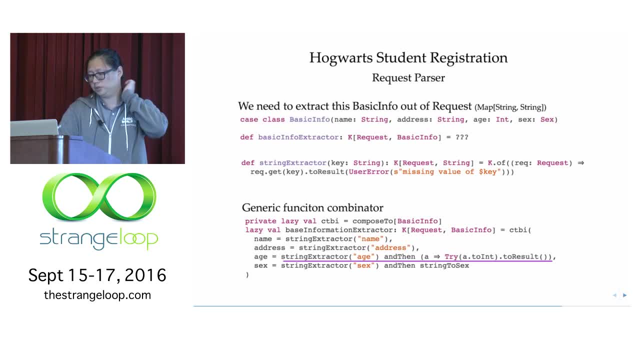 And we say: then what we want to do is to try to pass it into integer. We can just do that by using the second function And then combine them together using and then, And then we got another K of request to integer And then we can say: age equals to that. 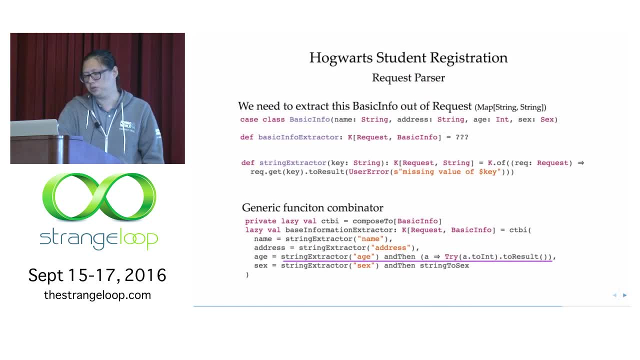 And then the last thing is similar to age, which is just, you know, to get the sex. So then the whole thing is a function of request to basic info. So, as you can see, you don't have bond variable here. 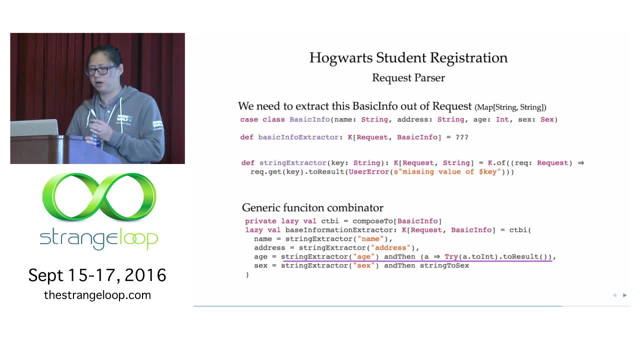 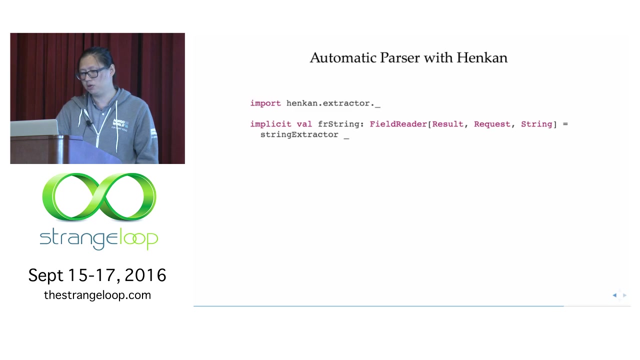 It's just, you know, you just combined multiple functions into a function. that That provides the all the relative information needed for the basic info. Still making sense, everybody Cool? So we can also do automatic parser with Hankin. 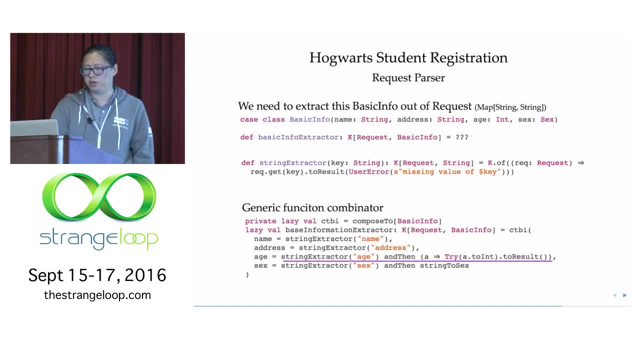 So, if you look at this, this is the manual parser. What do you mean by manual parser? Because you still have to compose So you can do basic information parser or extractor or K from request to basic information by providing name, address, age and sex. 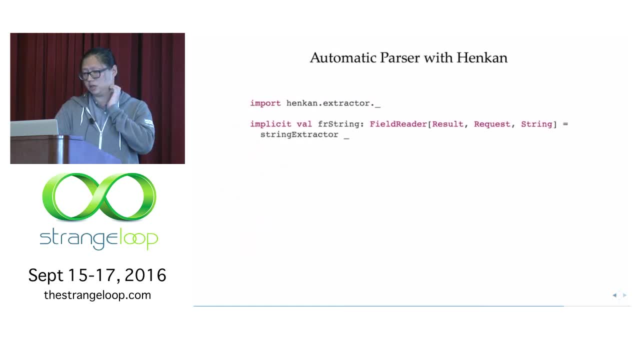 And all the functions do that. But with Hankinextractor you can basically provide a function that from the map to you want to say: give me the field, I want to get a string value out. So the first thing you provide is a way to get a string value out of a map, given a key. 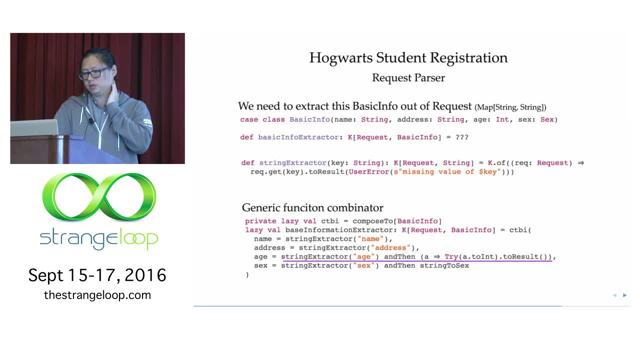 So that's basically string extractor. So that again you can see the string extractor here. Here I just you give a key and you give a function that you know, given a request, extract a string out of it. 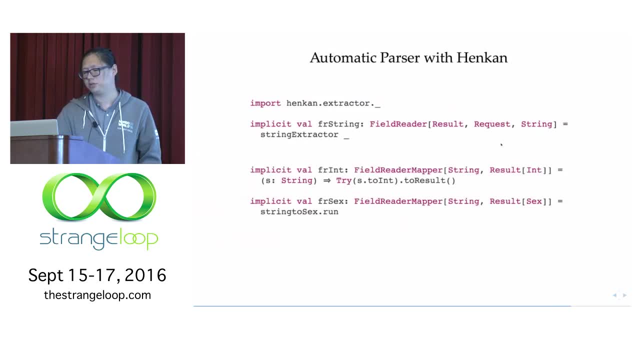 This is the first thing it provides. And then it provides functions that, Given a string, I want to get an integer, And given a string, I want to get a sex. So it's string to result of integer, string to result of sex. 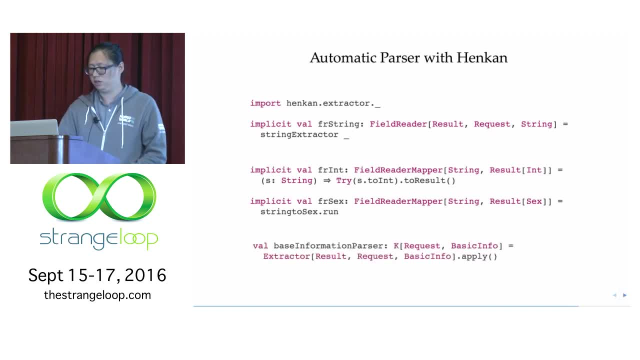 It provides all those implicitly in Scala. You can use Hankinextractor to automatically compose extractor from result to request. Sorry, from request to result of basic information. So it's K of request To basic information. Again, the K is just the function from request to a result of basic information. 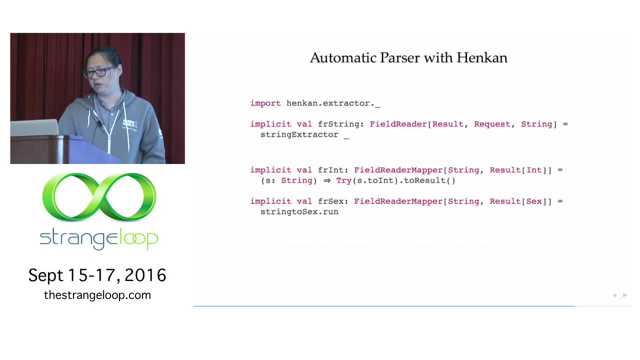 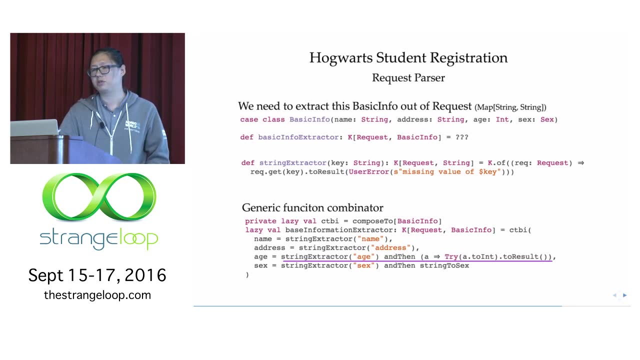 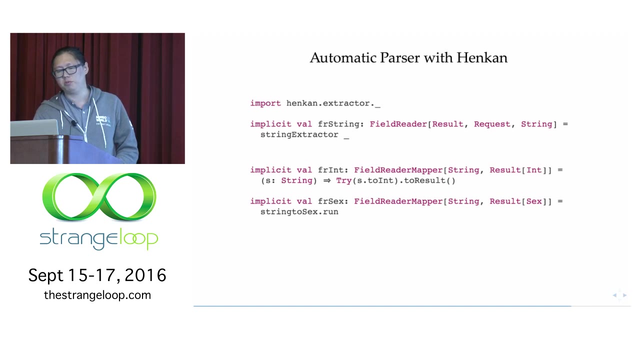 It just called this. It automatically composed that for you So you don't have to manually write you know: name equals slot, address equals slot. You don't have to manually combine those extractor into one And another thing that if you have a different data structure, as long as you provide all the primitives of you know the thing that you can convert in primitive types. 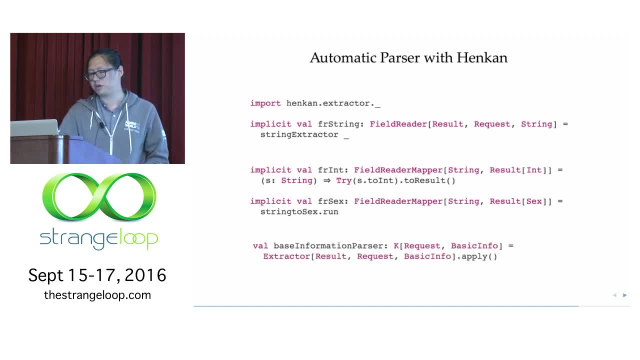 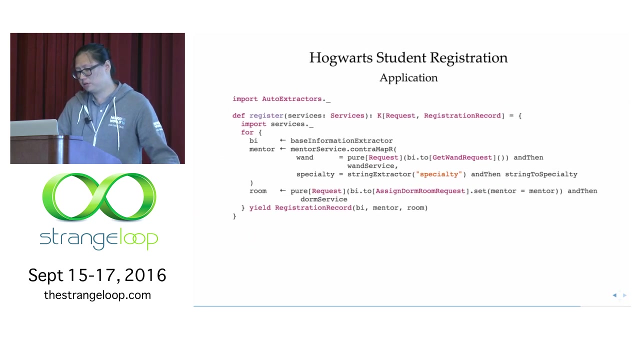 you can automatically get the extractor for that data type or presentation automatically for you. So that's automatic parser with should be automatic extractor with Hankin, All right. So now let's look at the final application Which we want to combine all the services I mentioned before, which is mentor service, you know, the Wend service which gives you a Wend. 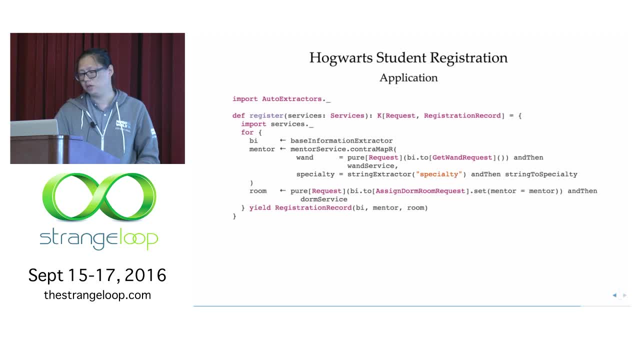 Mentor service assign a mentor for you and a dorm room service that assign a dorm room for you. So let's look at this. It's going to be quick. I mean it's going to be interesting, But I think it's as concise as can be. 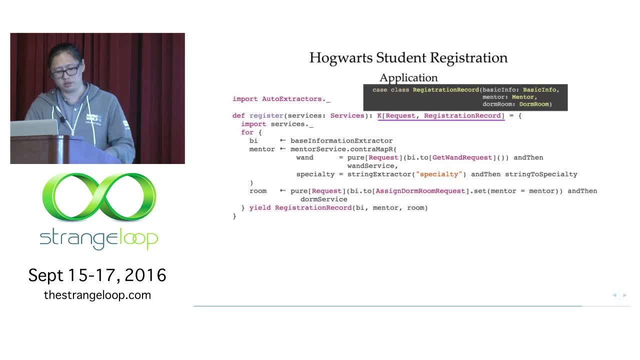 So what we want to build is a function from request to registration record. Just to remind you again, the registration record has basic information in it, a mentor in it and a dorm room in it. So we want a function from request to that. 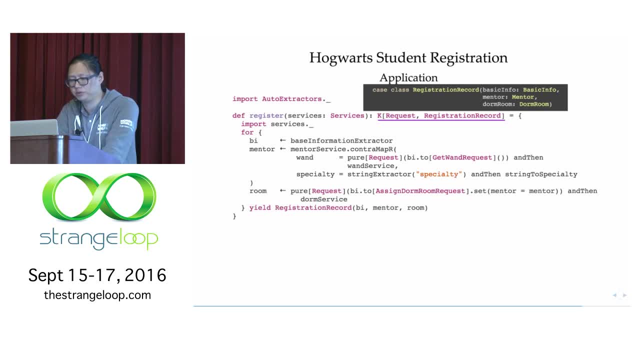 How do we combine function? How do we do that? So remember the whole thing. Each K is just a monad, So we can use four loops. This is how we do it, And the first thing we can get is the basic information extractor. 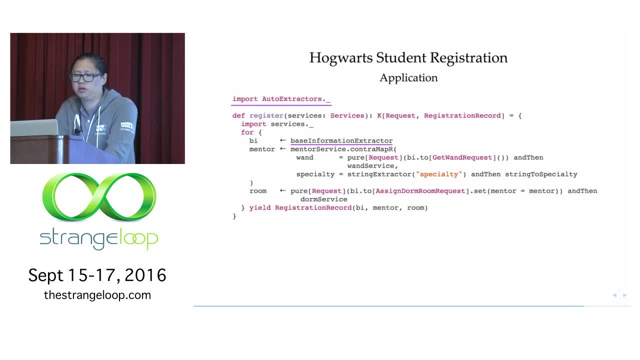 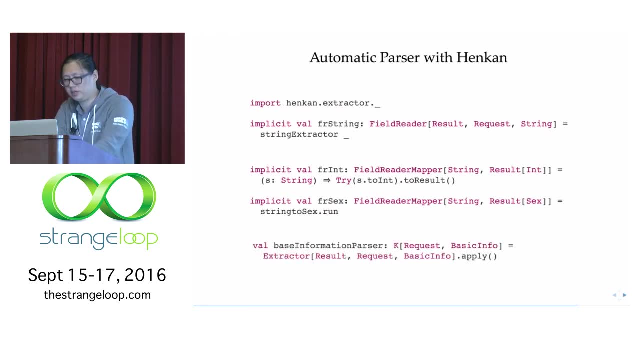 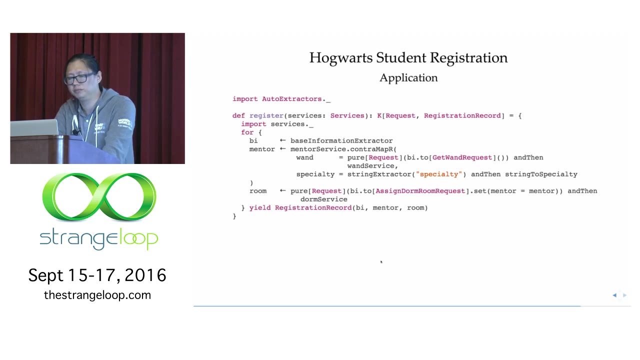 This is the one that we just constructed using auto extractor or the manual extractors. So it's basically this guy, This guy, The guy just appeared. We use that here And we get a basic information out called BI. So that's why it's from the auto extractors. 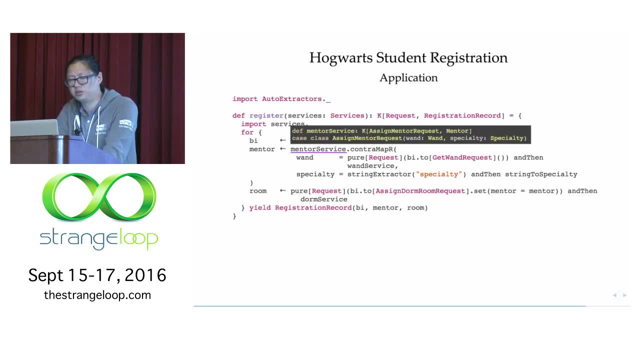 And then we need to use the mentor service to get a mentor. The mentor service, as you can see above, it requires a WAND and a specialty. So this is how we combine several functions into that mentor service function. We can say: the WAND is from: 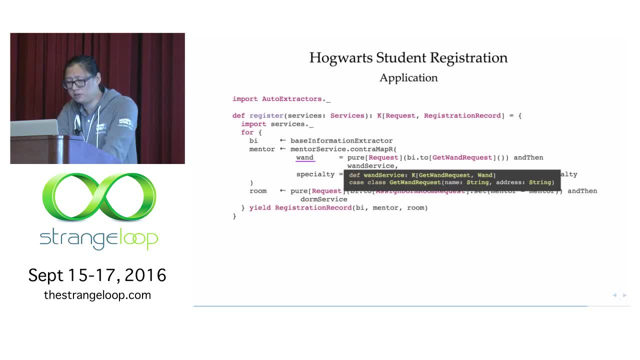 We need WAND service, So the WAND service in this turn needs name and address. Okay, Where do we have name and address? It's in BI, right? BI has name and address. The basic information has name and address. 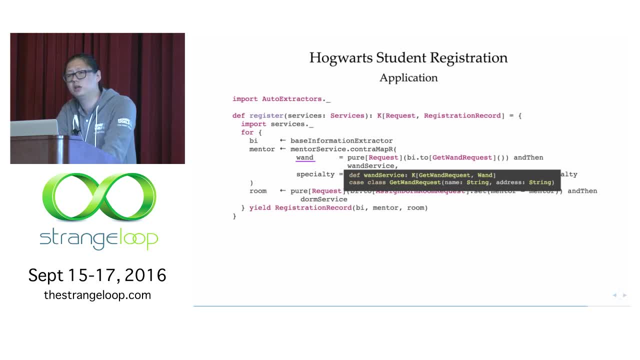 But in this particular WAND service it takes a different data presentation. It takes a get one request. It also has a name and address. So what Hankin does is provide a convert module That you can just convert from one case class to another case class. 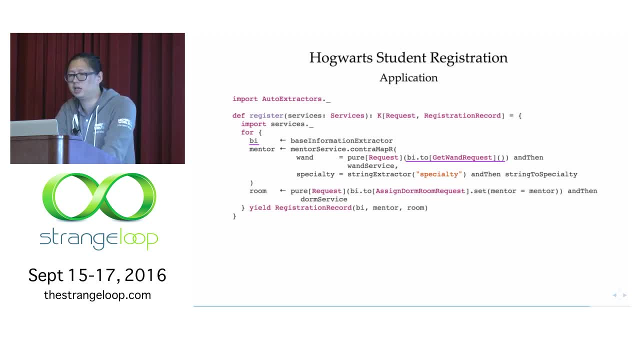 As long as the origin case class has all the fields the target case class has. So in this case it is this. So the get one request has address name and the basic information also has those fields. So you can just call two. 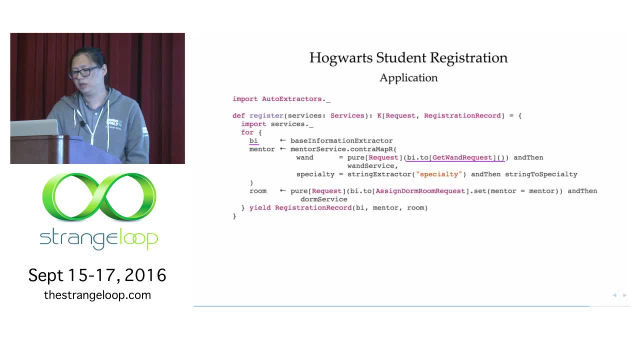 And now you got a get one request out And then you can call a pure request. This is pure. The key is classlypure, So it creates a classly out of a constant value, And then you call, and then 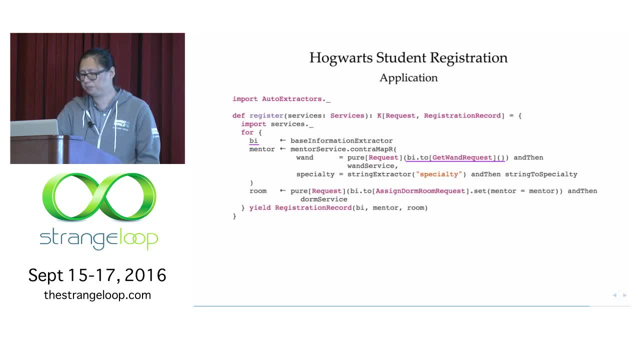 You combine that with WAND service, Right, Because now you have a classly of WAND request. Sorry, You have a classly of WAND WAND request, So you can just call and then, And then you got a classly from request to WAND. 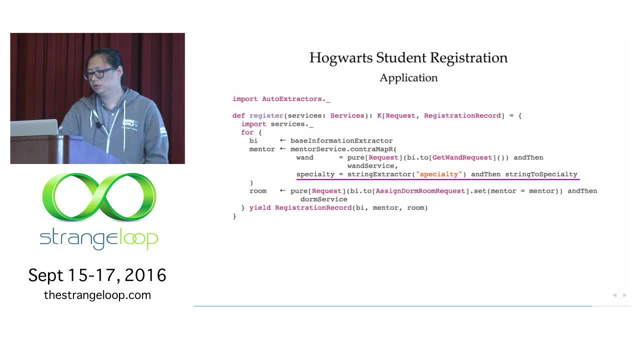 And then we want to get the specialty- The specialty is just going to come from the request, which is the map- And we use the string extractor again here, which got the value of specialty out of the specialty key, And then we can call string to specialty, which is a function: simply convert string value of specialty into enum of specialty. 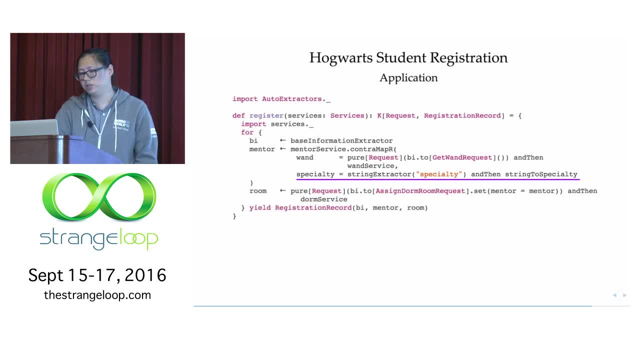 That's easy. So now, with WAND and specialty ready, we can call: the mentor service is ready, We call the control map R, which then is a function from request to mentor now. So basically, everything you see here is just K. 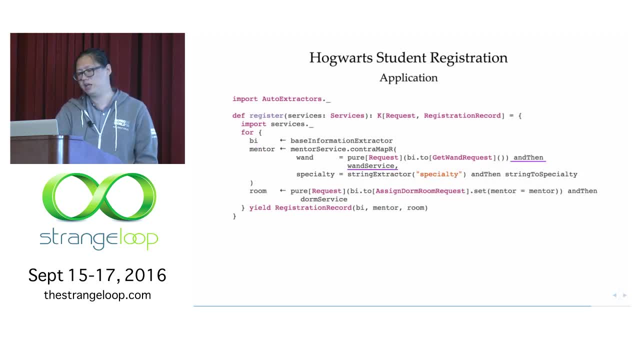 You see a K here, Then combine with another. K is another K, And here is another K, They. just when you call control map on them, they also are Ks. Everything is just K. So classlies, Then the final one is the dorm service. 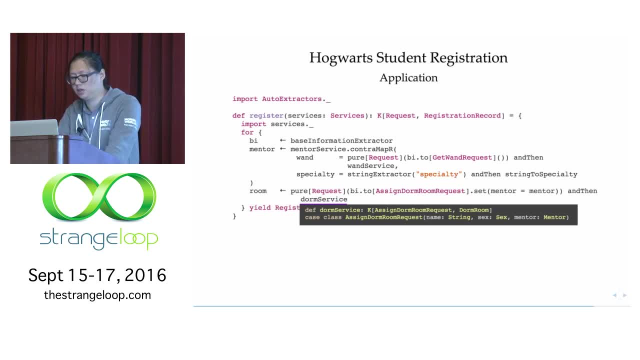 What we need in the dorm service, we can see, is string, sex and mentor, And so, again, we remember that name and sex is also valuable in the basic information, which is BI So, but mentor is not. So this is the case. 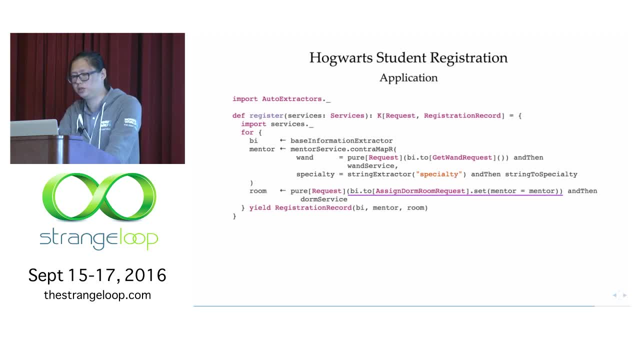 We want to convert a basic information into assigned dormant request which has both name and sex, but not mentor. To convert that we have to provide mentor. So we can call BIto this new request and call: set mentor equals to mentor. 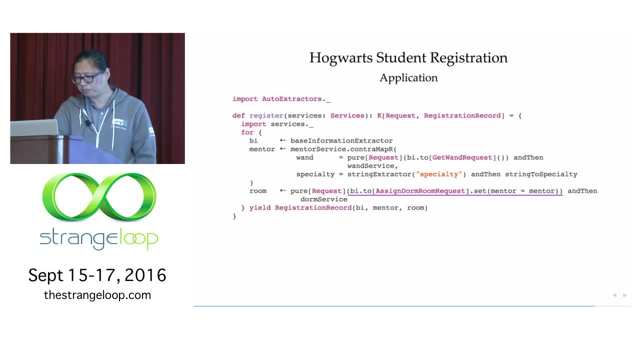 Now we get an assignment dormant request out. So this is another function provided by Hankenconvert. If you're trying to convert a case class to another case class but you don't have all the fields that the target needs, you can just manually set it in the set function. 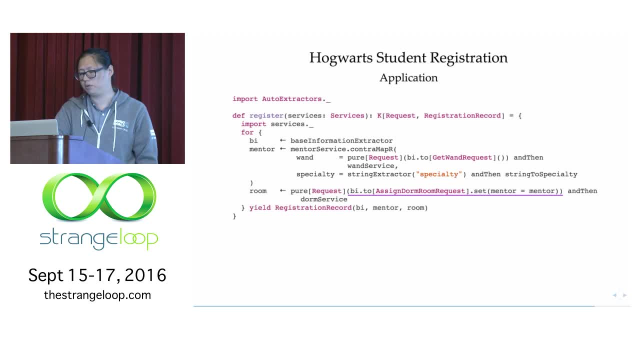 So now you have assignment, dormant request, case class, And then you call that. You got the function. You just combine this to the registration record. Then you got a function from request to registration record And it's a combinator of all these functions. 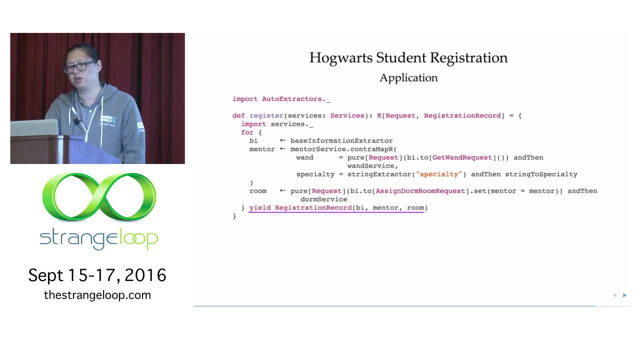 With some, you know, Hanken, conversion, you know kind of like glue between the data presentations needed by those. So voila, you have the final product And we don't have, I don't, we don't have much many.